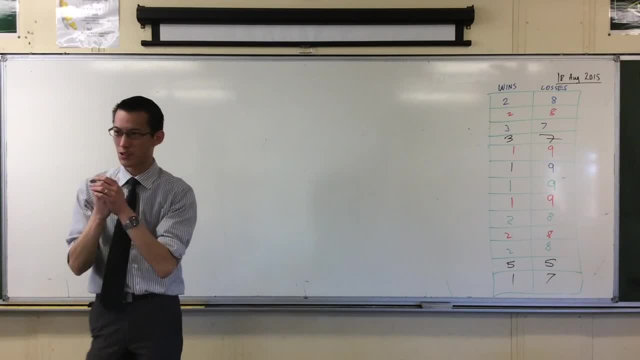 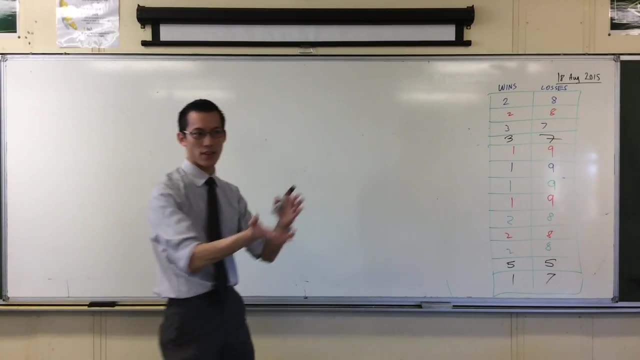 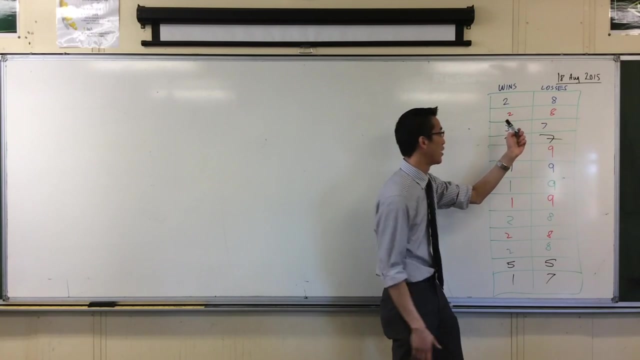 Hi, I've asked some people to add up some numbers for me so that remember, at the beginning I asked you to make a prediction about whether you thought like: was the chance very high, very low as a percentage, what was your chance of winning and escaping Voldemort, rescuing everyone, or what were your chances of getting killed? okay, 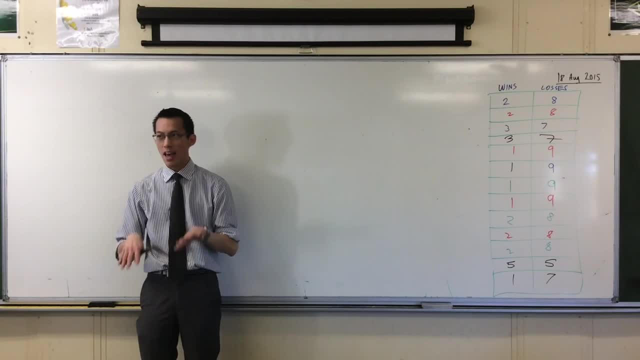 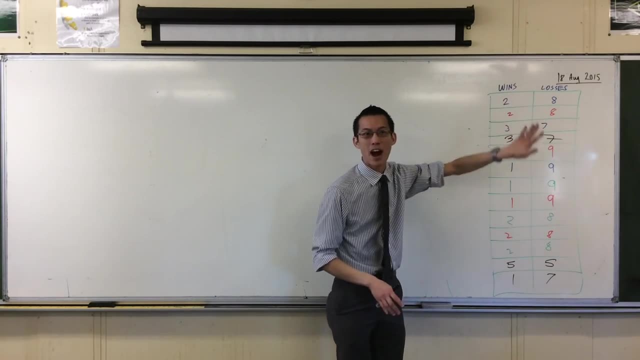 Now don't actually say it yet, but who reckons they have the highest, that is, the most optimistic percentage for the number of wins? Who thinks they have a very high number? Anyone, Anyone. Okay, Jordan, what's your number? 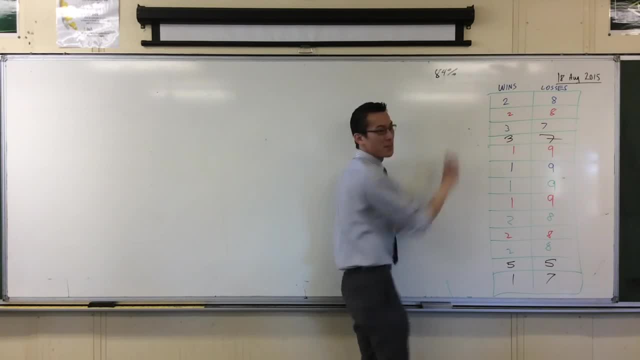 84%, 84%. Anyone want to beat 84?? 90%, Okay, As a chance of winning, right Chance of winning. We only win once. We only win once. We only have to end the win once, so it's like one roll. 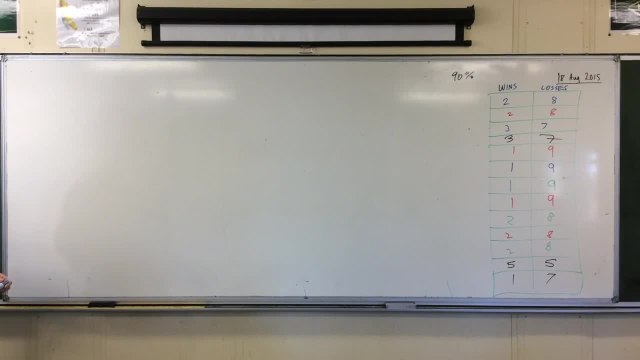 Oh, once out of the ten, Once out of all ten. Ah, no, no, so you misunderstood a little bit, Just like when I was talking about flipping right. It's 50% every time. 50% every time. Does that make sense? 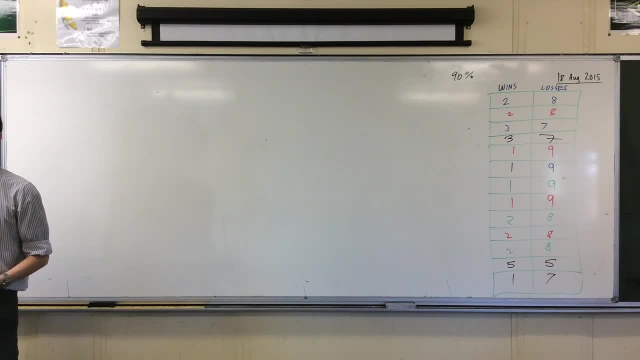 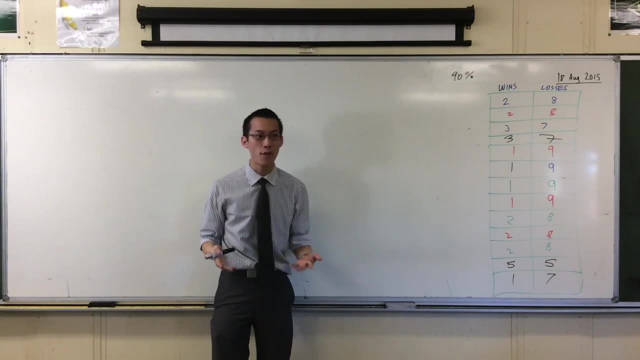 Okay, who reckons they're a bit of a downer? had a very pessimistic who reckons they had the lowest number. Okay, Tendai, what did you think? 40%, 40%, Anyone go lower than 40? Nathan. 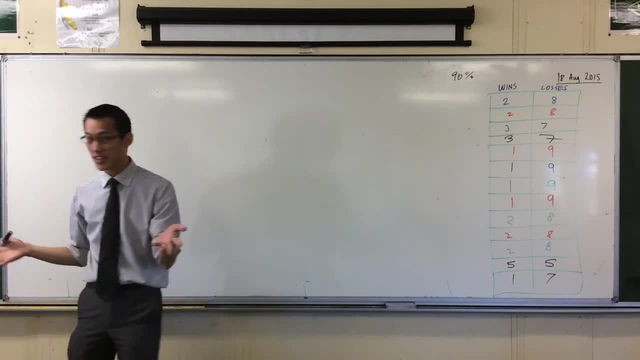 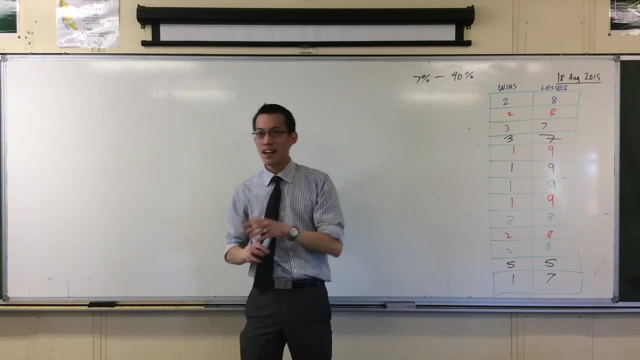 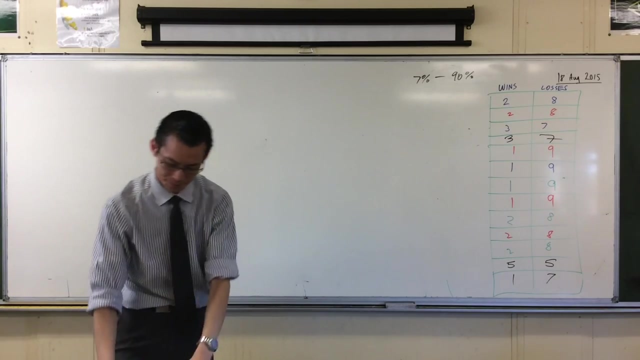 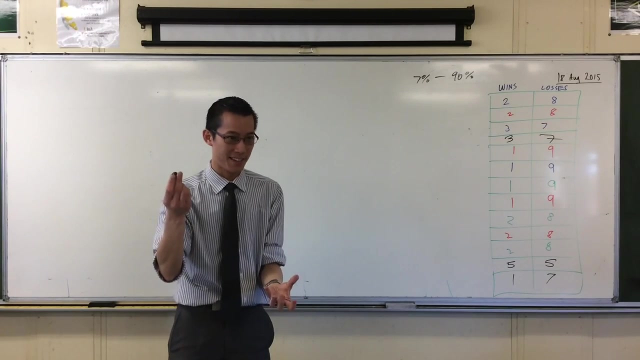 Seven, Seven percent. Anyone go lower than seven. Eight, Seven, Seven's our lowest number, Eight. Okay, now can I just say this thing here: what you just did, right. In some senses, this might be one of the most important lessons that you learned today, namely this idea of remember. we said probability, the name of the topic is probability, but it's really about chance and uncertainty. okay, 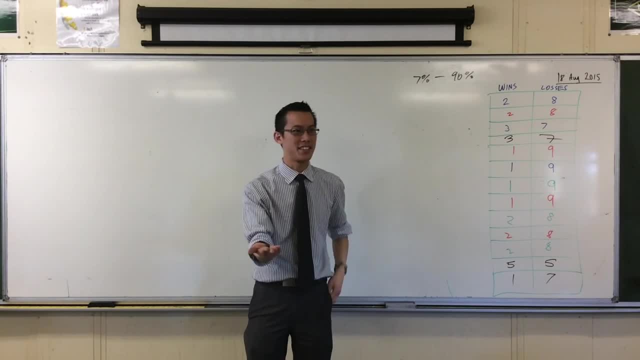 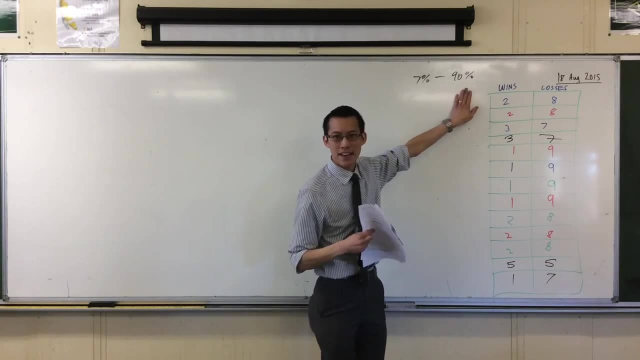 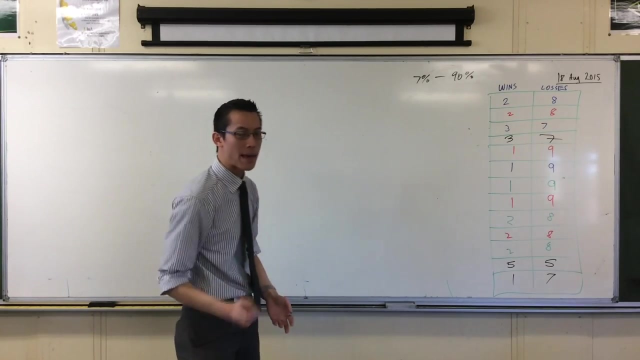 We live our lives every day with chance and uncertainty. It's not as neat as a die. In fact it's more like what this game is like, where look at the range of essence And I assume we have everyone in between, okay, And that's kind of what life is like, right, Like you're not sure what's going to happen but you have to make an action nonetheless. okay. 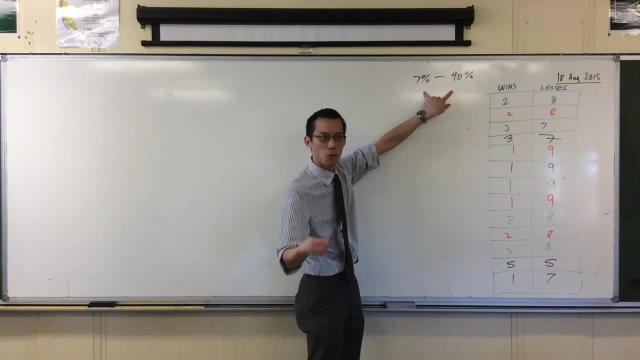 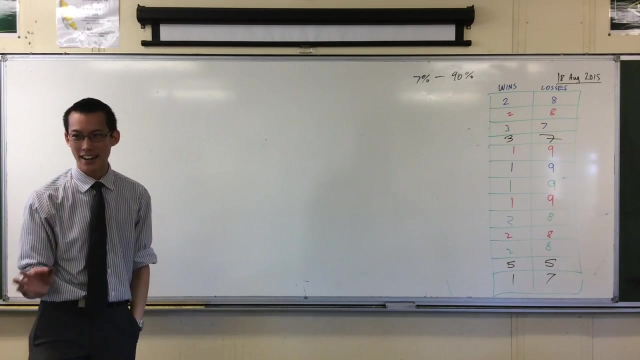 This idea of estimating the chance that something will happen, right. This is a really, really important numerical skill, right. So that wasn't just a cheap shot, right. It was actually something really valuable to do. And here's the thing, right. We have data. now it's on the board to actually work out. 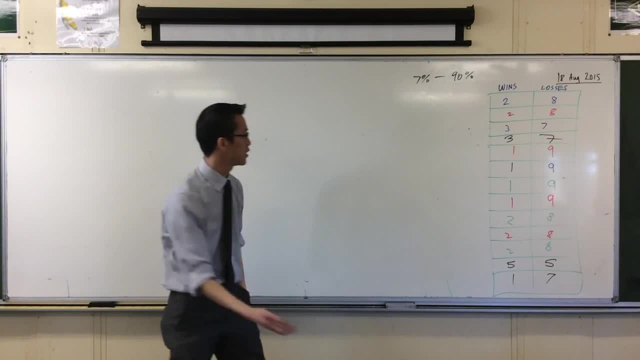 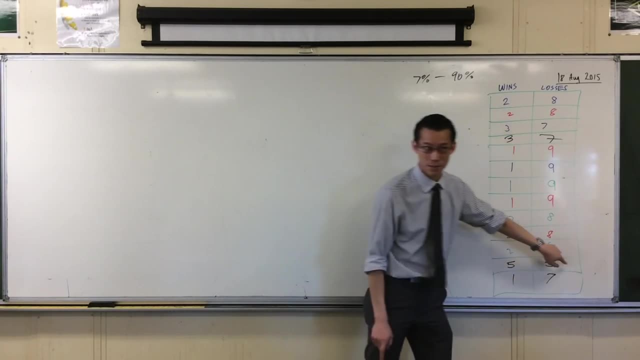 To actually work out a percentage, because, based on yours, for instance, if I was just: this is Kyle, this is you right, You're Daniel, okay. Now, if I just played this number of games- 10 games, right- What would you conclude is your chance of winning? 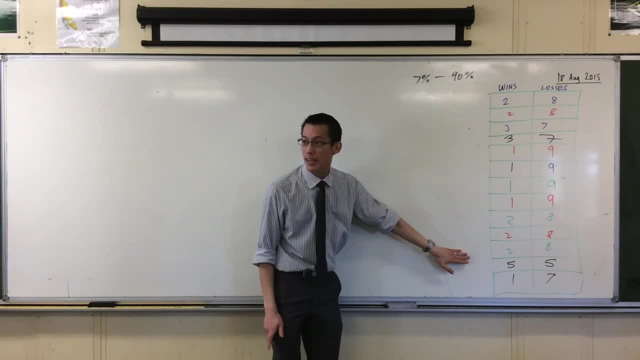 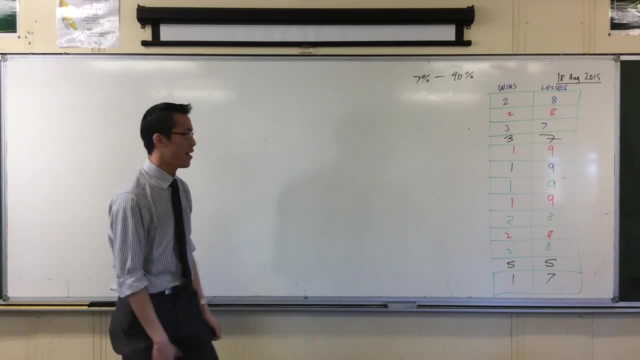 50.. You'd assume it's 50-50, if that's all you've seen, right. I'm glad there's no one here who never won, ever right. But suppose you played the game and it's like I never won. I just lost 10 times in a row. 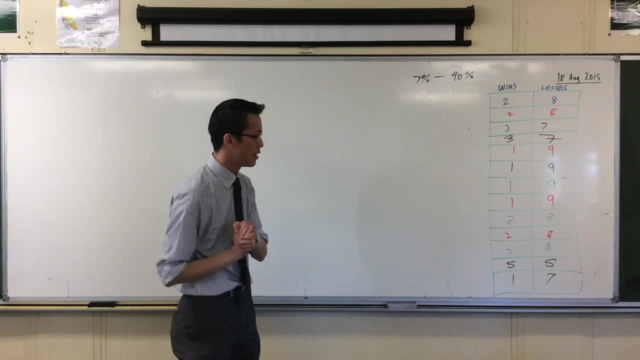 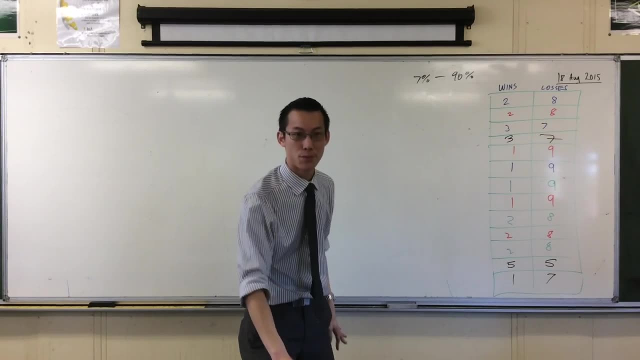 It wouldn't be that unreasonable to assume that the chance is what. It's impossible, or at least it's less than 10%, something from a very, very low. So I asked some people to prepare some numbers for me. Daniel, how many did you do wins? You added up wins, right. 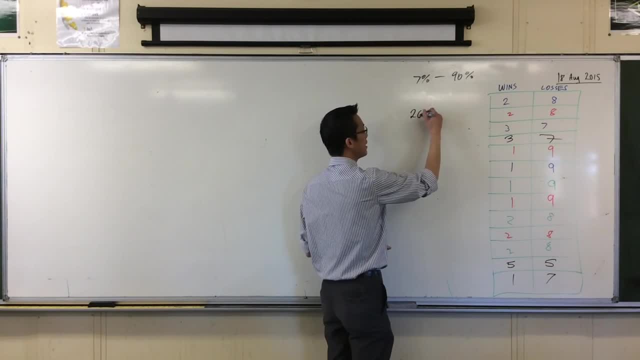 How many wins in total are there on the board? 26.. 26 wins. okay, Mr Hughes. number of losses: 102.. 102 losses. Okay, now pause for a second. I'm interested in a chance. 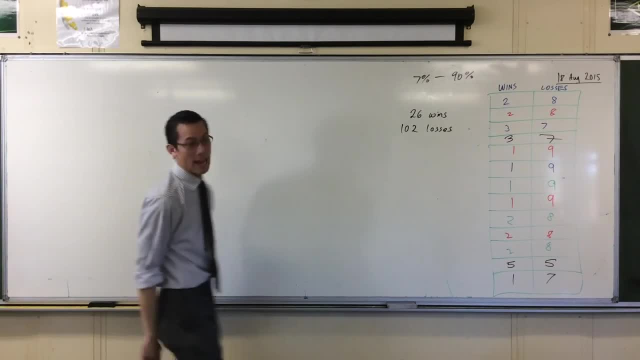 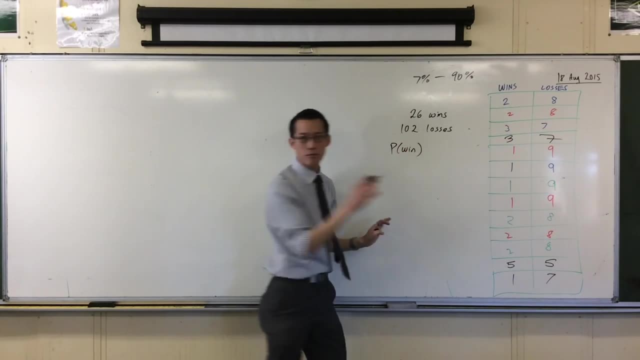 I'm interested in a chance, a probability, right? I asked you about wins, not losses, even though they're kind of the same thing, right? So wins, the probability of a win, through this experiment that you guys have just done and collected the data, the favorable outcomes are 26.. 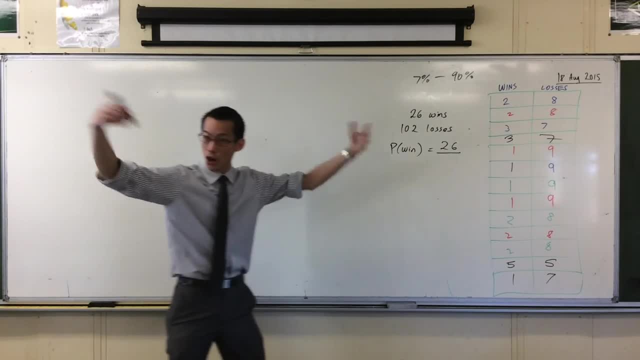 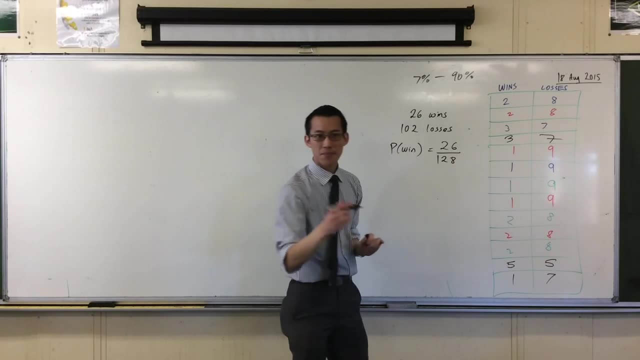 What goes on the denominator 125. It's going to be the total sample space, the number of times we play games, which is 128.. Yep, So I'm going to ask for a percentage, right? Can someone give it to me as a percentage? 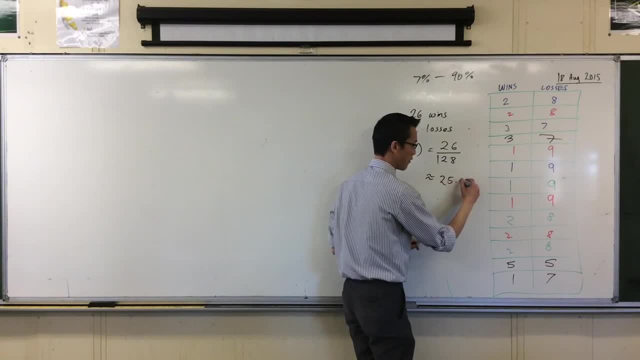 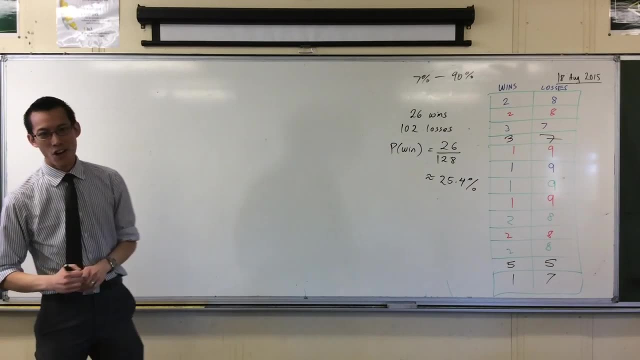 25.4.. 25.4? That's a nine. We'll just go four. okay, 25.4%, all right. Who reckons they got closest to that number? Rachel, what did you get? She got 25%. 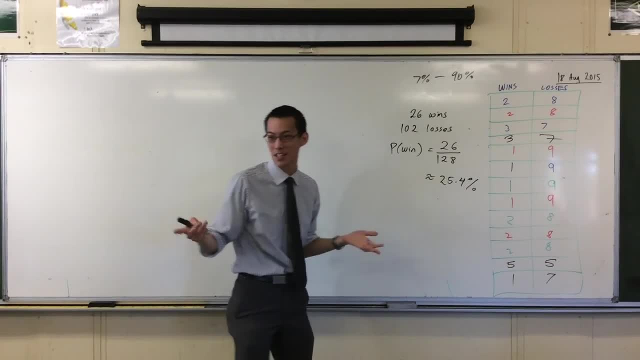 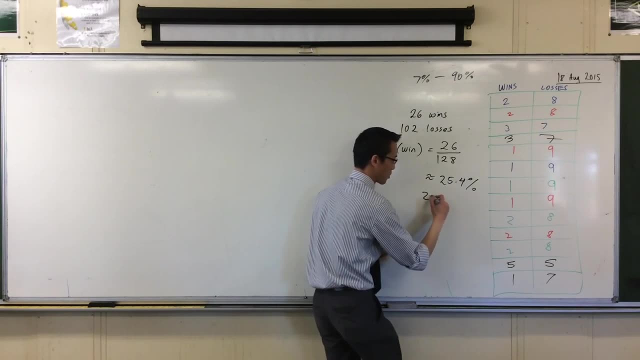 20%. Anyone think they got closer than 20?? She got 25%. 25%, that's if you. yeah, that's right. If you didn't do decimal places, that's the closest you can get. 25% is our closest estimate. 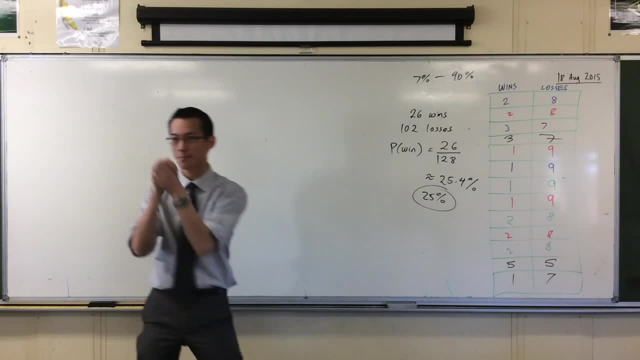 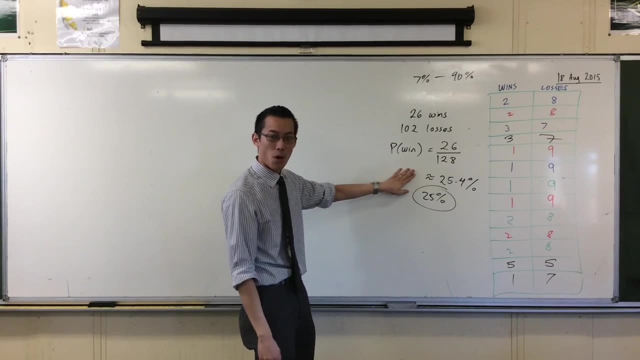 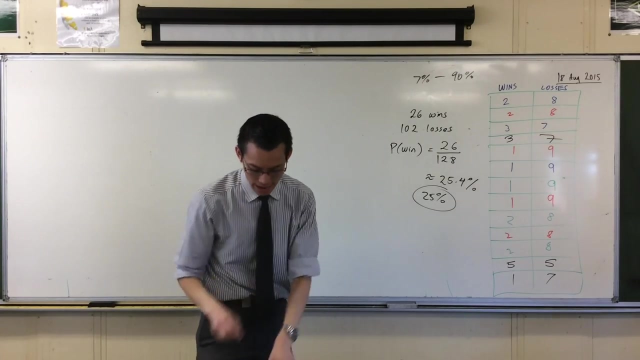 Oh, That's our closest estimate. Now stop for a second. I want you to look carefully at your number. Look carefully at this number. Were you too high, too low, and how did you arrive at that number? Okay, I'd like you to make a heading which is complementary events. 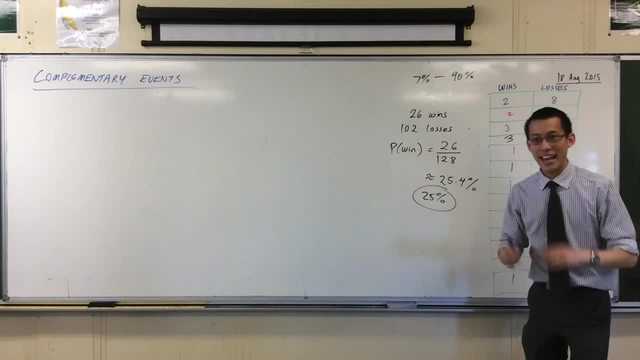 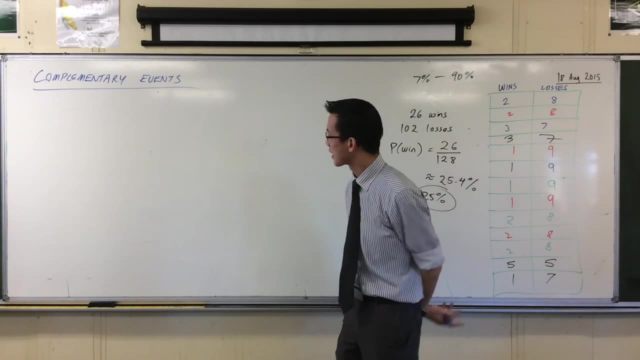 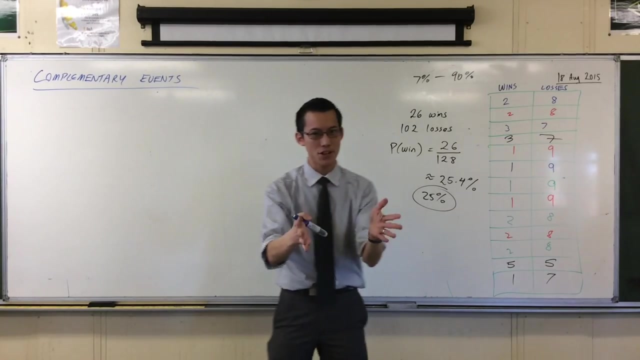 Okay, Now we're going to start to get towards this number, but we're going to introduce this idea, which is really just broadly useful. okay, You've met this word before complementary. You met it when we were doing a bit of geometry, right In geometry. if I have an angle like this, okay, 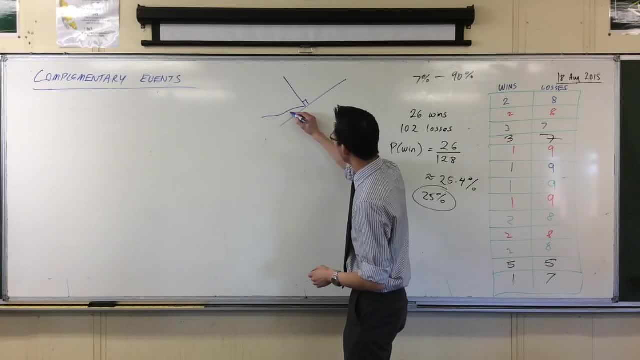 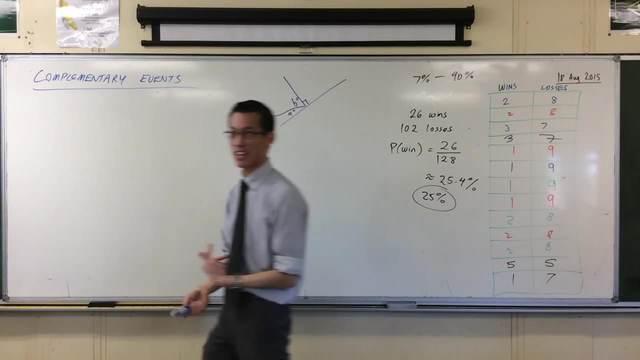 I have a right angle in there and then I've got some weirdo wiggly angle over there. A and B- Okay, Okay, Right, You know that A and B, when you add them up together you're going to get. 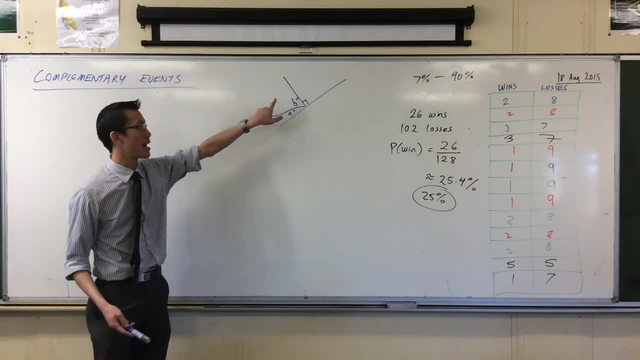 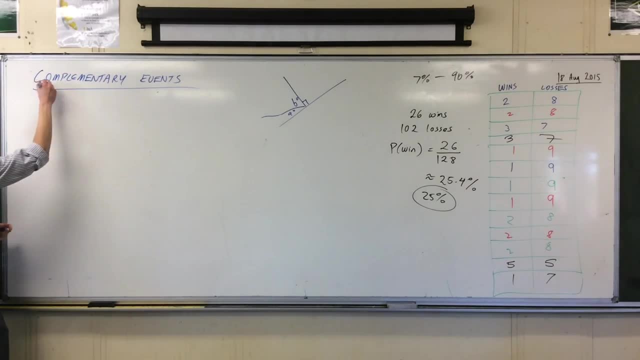 90.. 90 degrees, because the right angle on this side. there must be a right angle on this side, right? So we say A and B are complementary. Now, that's just really a general term Complement. please spell it with two E's. by the way, When you spell it with an I, that's like nice haircut, okay. 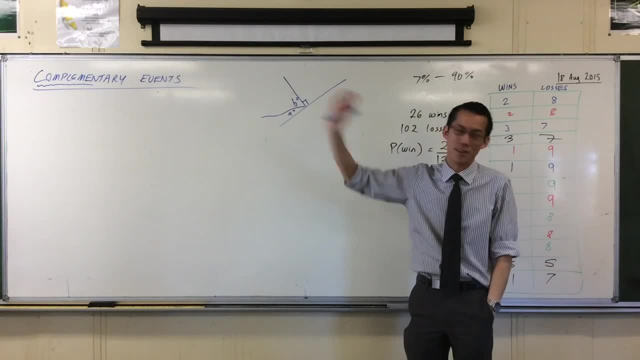 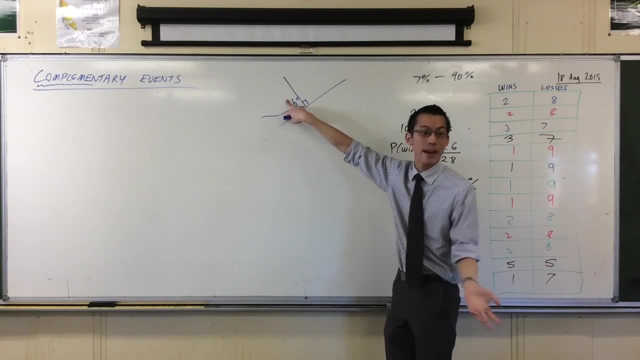 Complement. this is a com. I don't know. The pronunciation is the same. honestly, It just means things that go together, things that go together right. So these go together, they make a right angle. That's what complementary means in geometry. 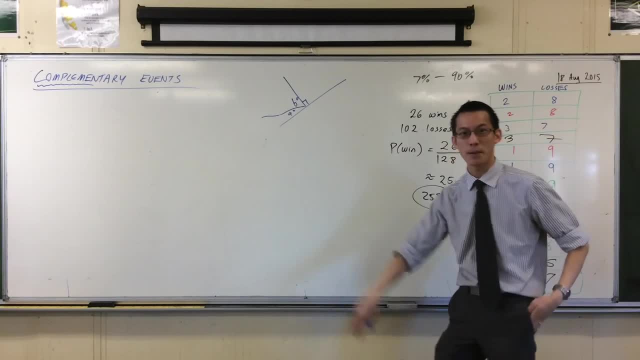 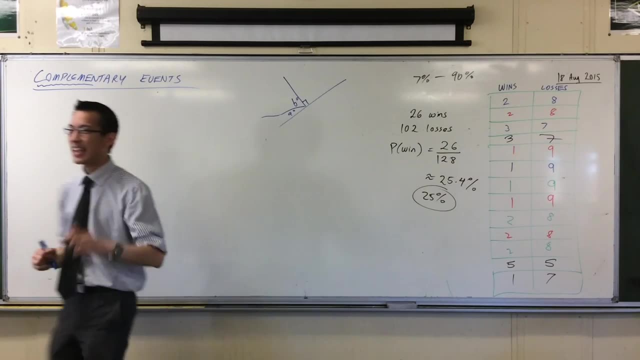 If your parents or you are like foodies and that kind of thing, they talk about complementary wines. A wine goes with a particular kind of food. It just means they go together In probability, right. complementary events are again events that go together. Here's the way I'm going to illustrate it, right. 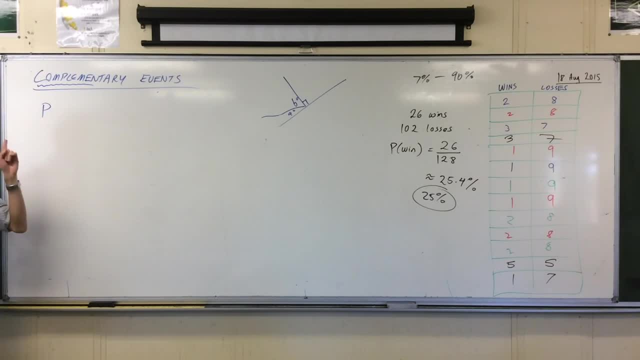 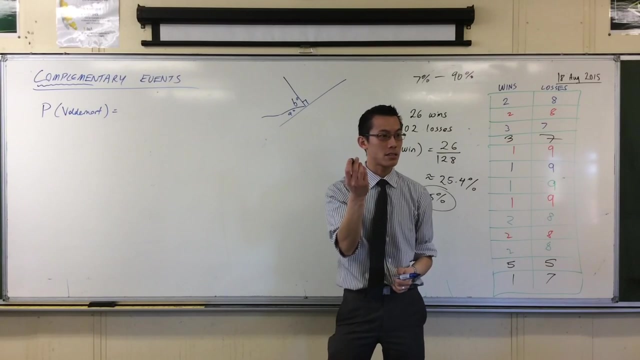 Underneath here, when we play this game, we can work out pretty easily on any individual event In any individual role. what's the probability of getting killed by Voldemort right? We can know this right because on the die there are six faces right And Voldemort is one of those faces. He's the sixth right. 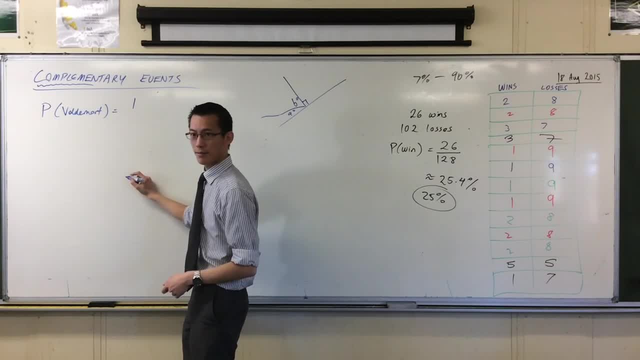 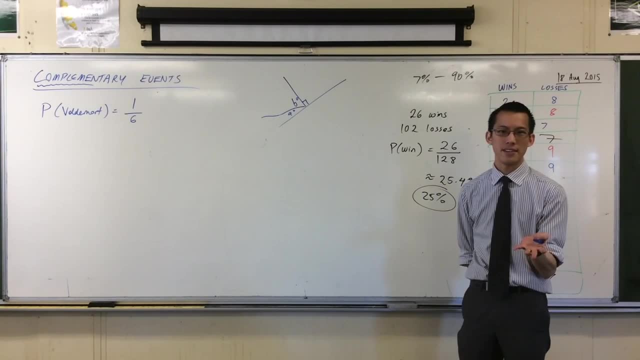 So we would say this outcome is one out of six. Go right, Sorry, one out of six. One out of six, Six faces on the die. So then I would say, right, as you were trying to roll, you were trying to do the opposite of that. 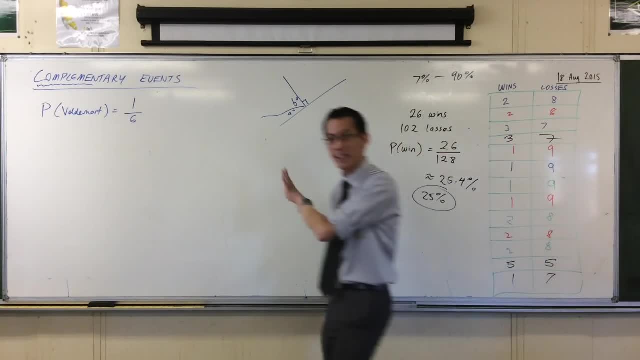 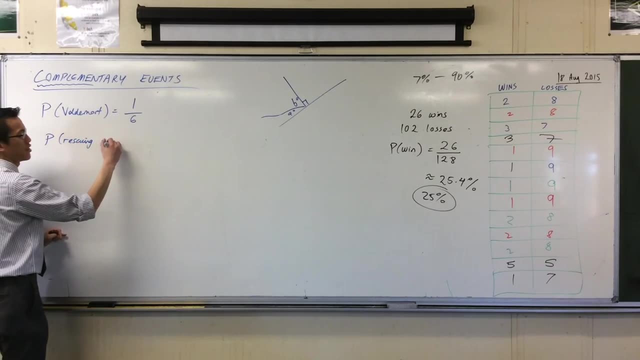 You were trying to do something else. You were trying to rescue someone, right? So I could say the probability of rescuing someone, and I'm just assuming you know when you first roll and not worrying about the fact that if you've rescued someone you can't rescue them again. 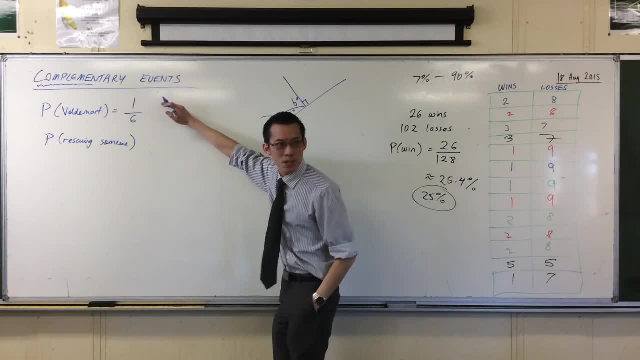 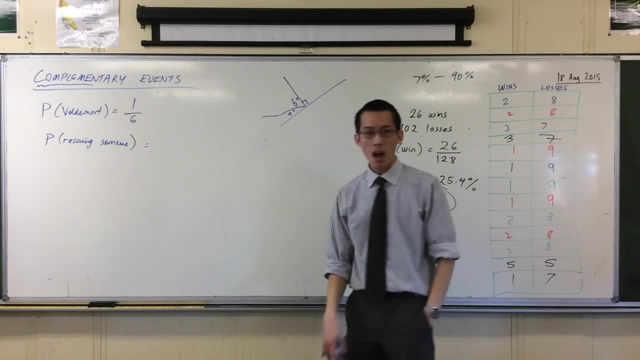 Don't worry about that. It's simply the opposite of this right. It's not one out of six, It's five out of six. right Now, just before you write five out of six, before you write five out of six, I want you to see that either this event, 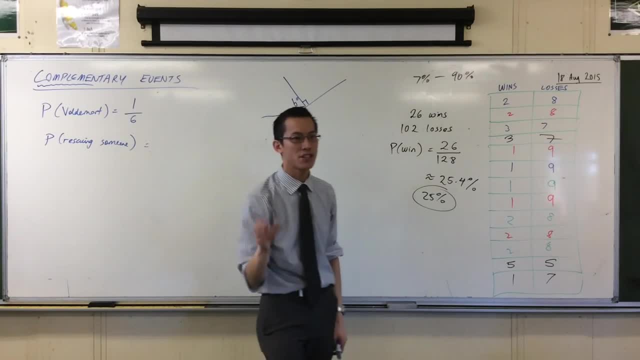 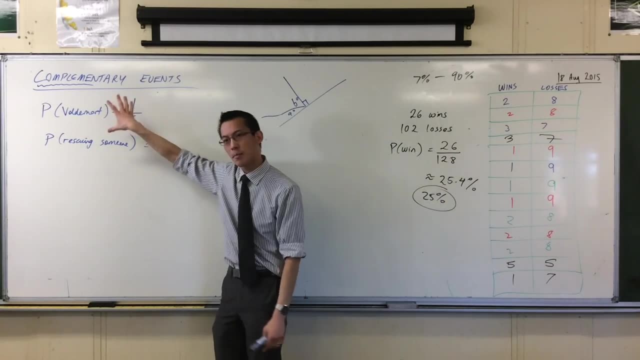 or this event. one of these has to happen every time you roll right. I mean, like I said, you know you've rescued Hagrid, you've already rescued him, but you're not dying right, So one of these must happen, right. 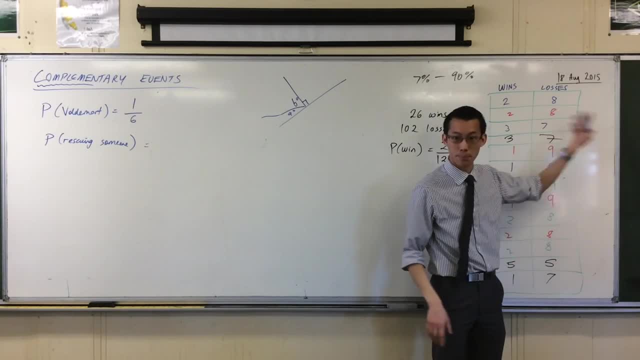 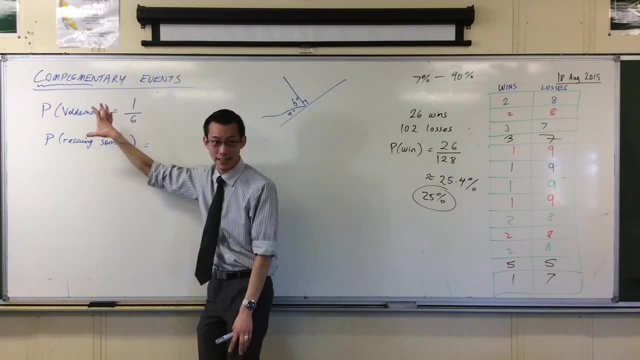 In other words, thinking back to the words we had over this side of the board, right, One of these is certain, or definite, or sure. You will definitely have one of these. So, therefore, it stands to reason that the probability of this, probability of this, if it's certain, it should add up to: 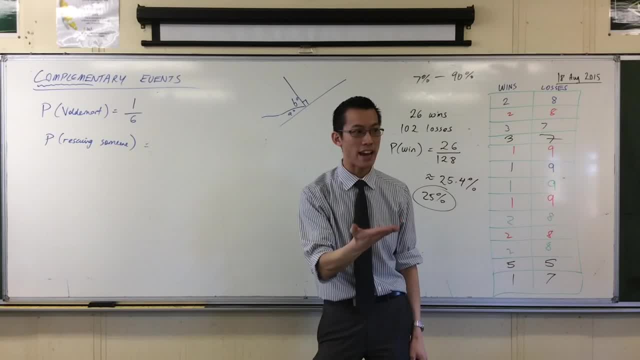 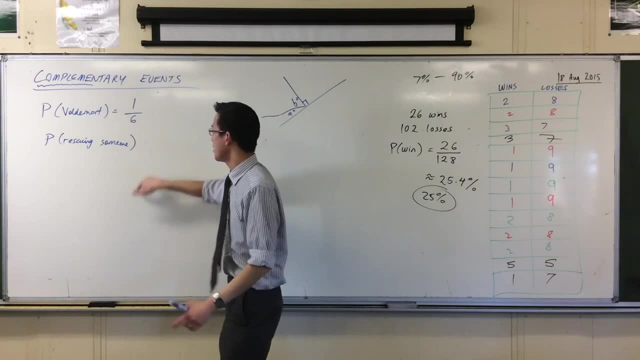 it should add up to one, right? Because it's certain A hundred percent chance, right? So I'm going to write the probability of rescuing someone plus the probability of getting killed by the other one. That's equal to one. 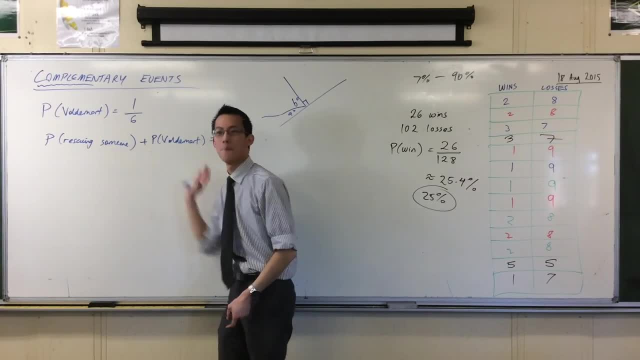 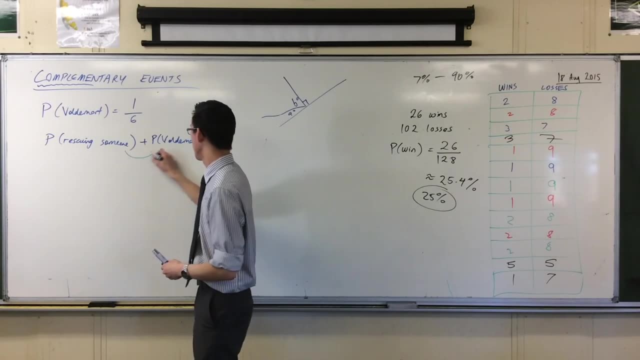 These definitely have to happen, right, One or the other must happen, for sure. They're opposite events, right, They go together And that's why we call them complementary events. They're complementary. okay, They're complementary because one or the other must happen. 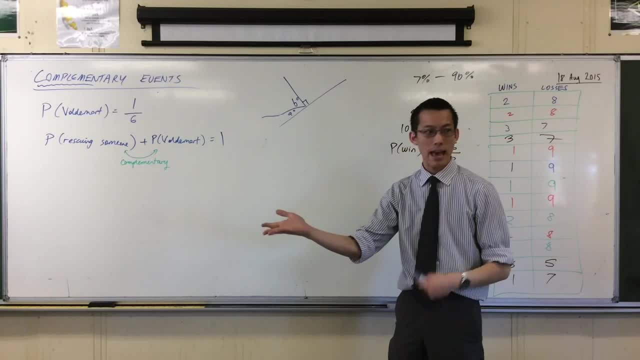 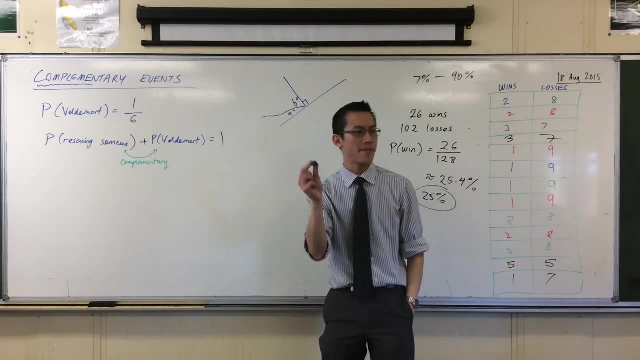 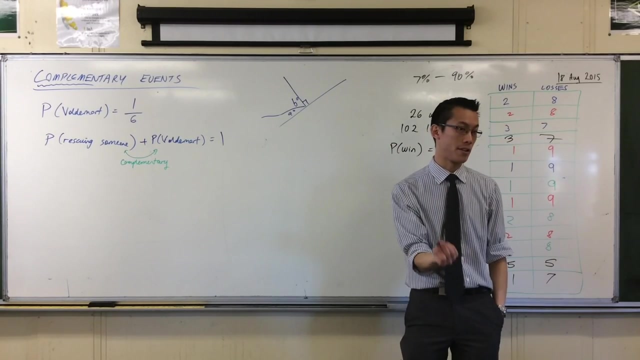 Going back to flipping coins: right, Heads and tails are complementary events. okay, Now come back to the diagram. right, Let's think of, say, five and six, Rolling a five or rolling a six. Rolling a five or rolling a six are not complementary events, right? 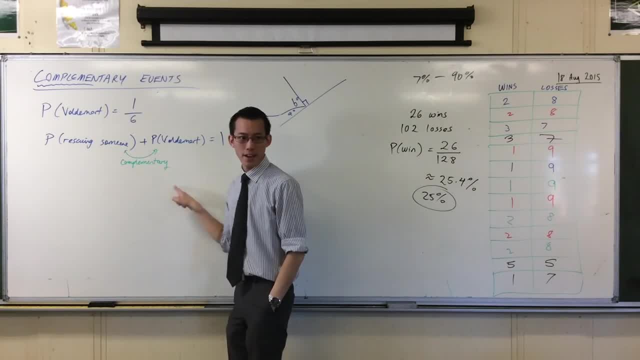 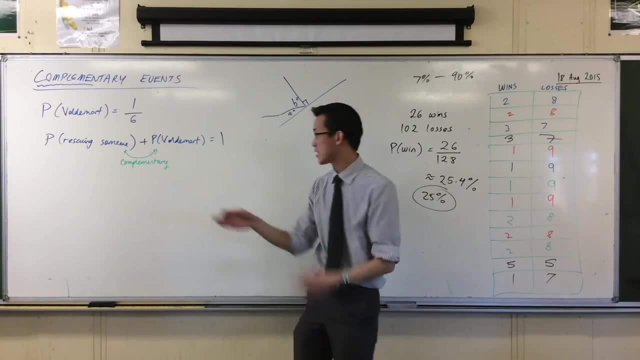 They are different but they're not complementary, Because you know what? I could just roll and sure enough I got a three right. It wasn't a five or a six right, So getting a five or a six is not certain. 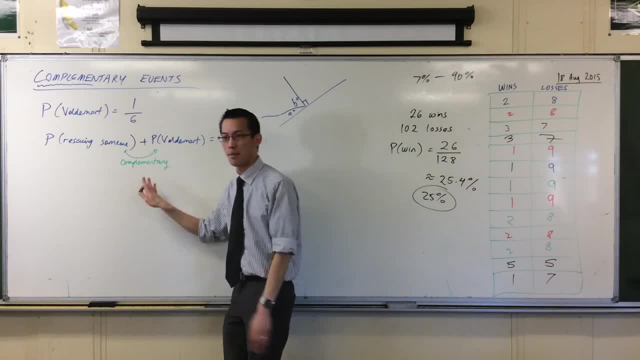 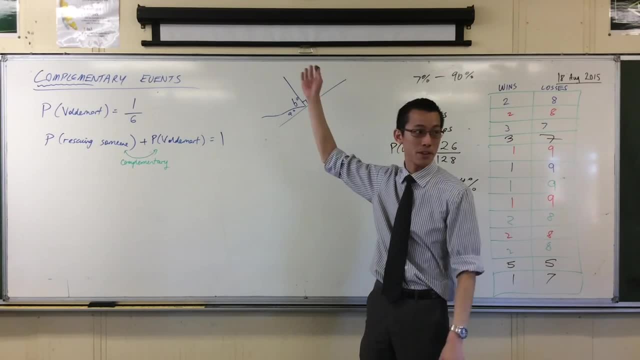 It's just part of it, right? So for instance, complementary, it's heads or tails, Voldemort or rescuing someone. They're the things that go together. Hence complementary Question: Does that mean that if you had, I'm sort of getting into a drama. 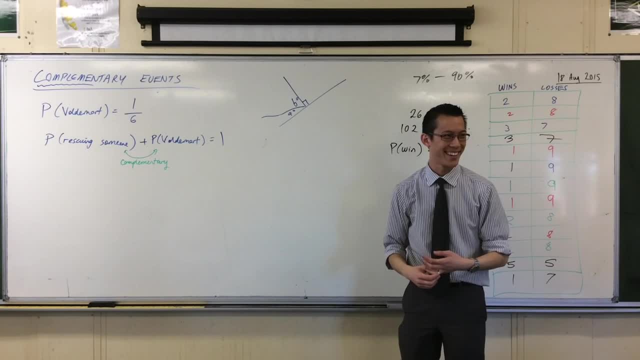 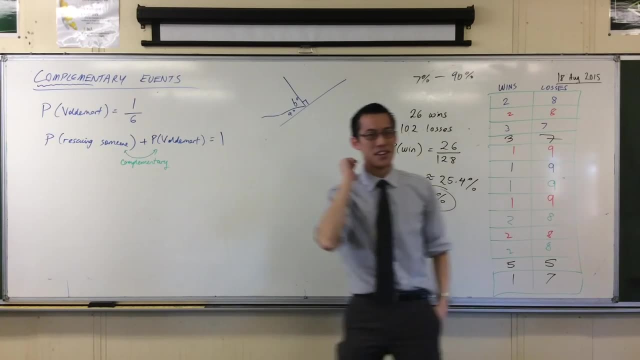 Yep, That geometry there. Yep, You get a supplementary. Ah, okay, So it's funny. Yes, you're right. I mean we tend to match those two ways together. As far as I know, supplementary doesn't really have a meaning in probability. 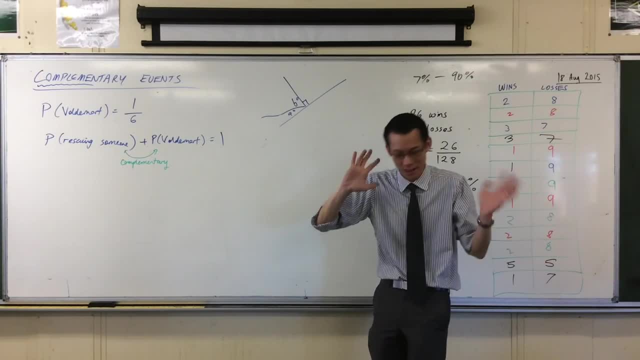 I think they kind of they use this one up and they're like: yep, we don't need another one. I guess, okay, But that's a nice thought, okay. Now, I'm going to finish this off now, right. 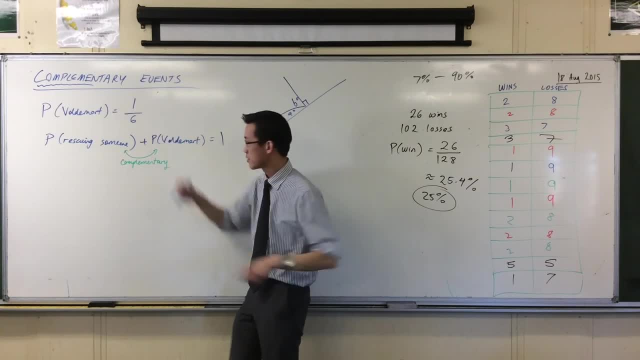 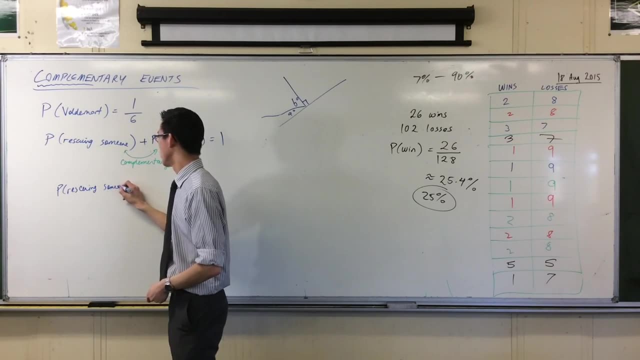 Because you already know what the probability of getting killed by Voldemort is right, So I'm going to write this like. so, Just going down to the next line, The probability of rescuing someone, plus this probability, which is just a sixth. 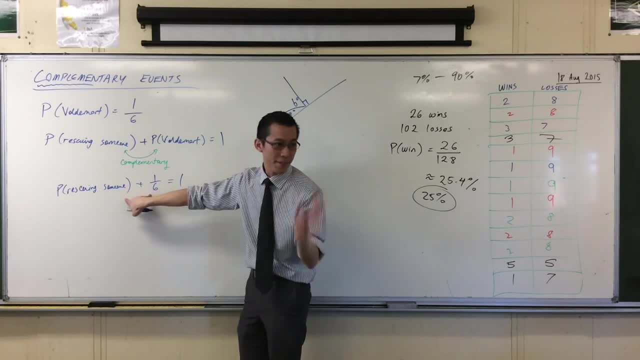 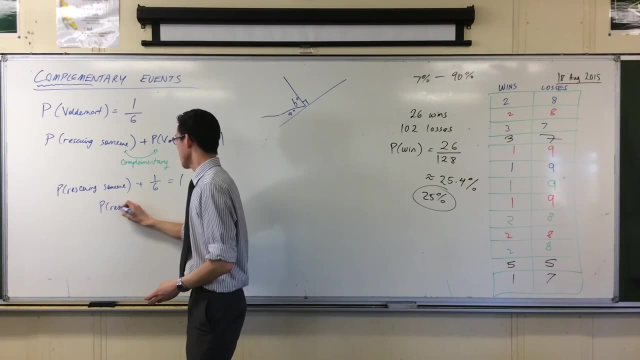 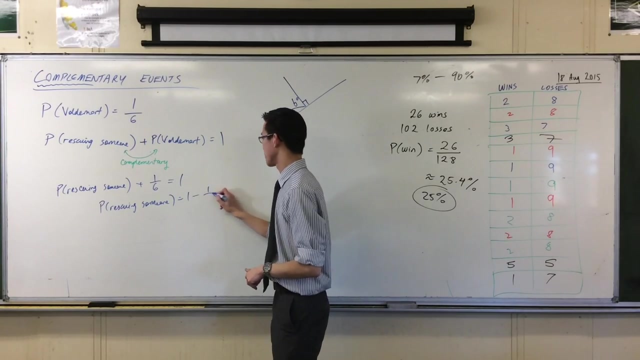 that should equal one right. One of these definitely has to happen. That's why it's a one. So now just rearranging That probability of rescuing someone. if I take that one sixth over to the other side, that's what gives me the five sixths that you were already expecting before. 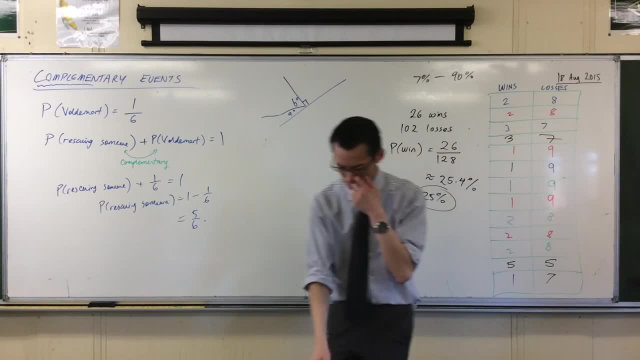 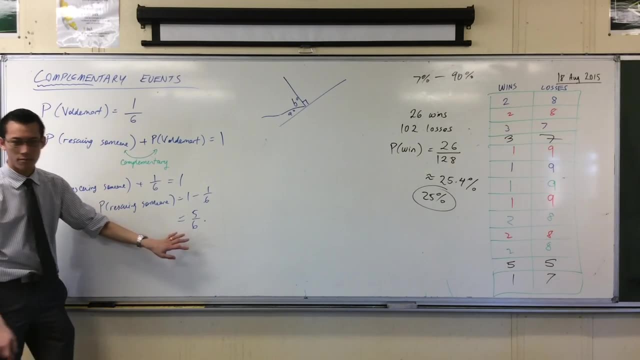 Okay, Now I've got a question for you right? Quick rhetorical question. If the probability of rescuing someone is five over six, that's quite high. If you crunch the number in your calculator, that's like 80-something, right. 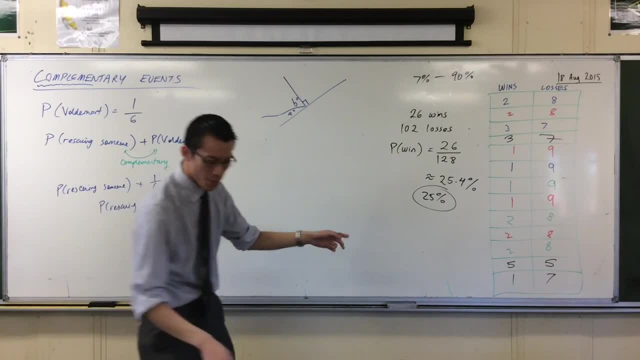 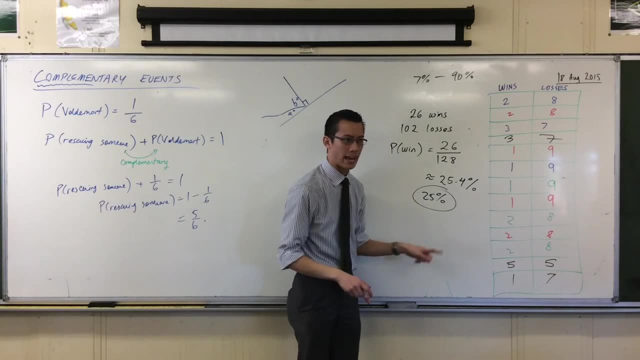 That's why we've got 84%. Ah, 84%, okay. So why is it? if this is 84%, why is it that the probability of actually winning the game is not 84%? Daniel, what do you think? 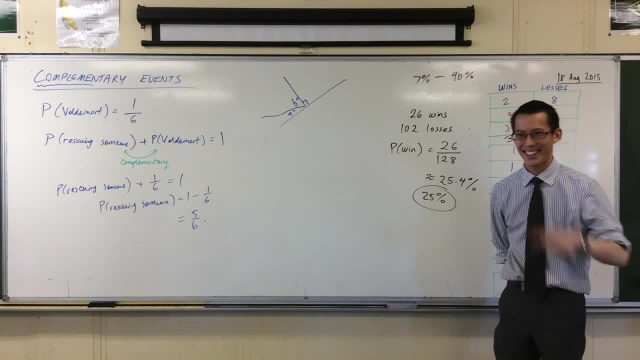 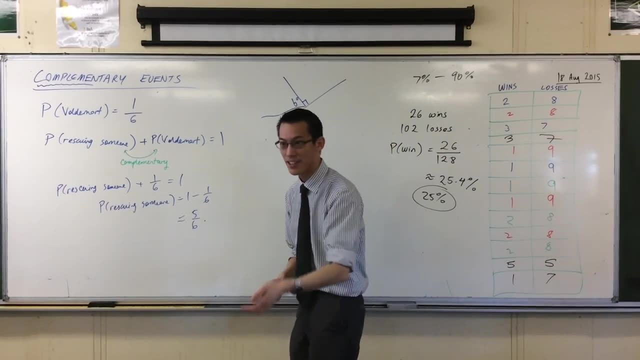 Um, because each number is one out of six, Yep, Which means you have one out of six chance to get like one in three. Yes, very good, That's right. So you see right The reason why this 84%. 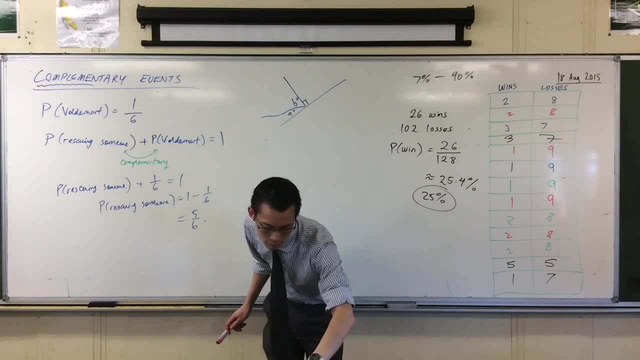 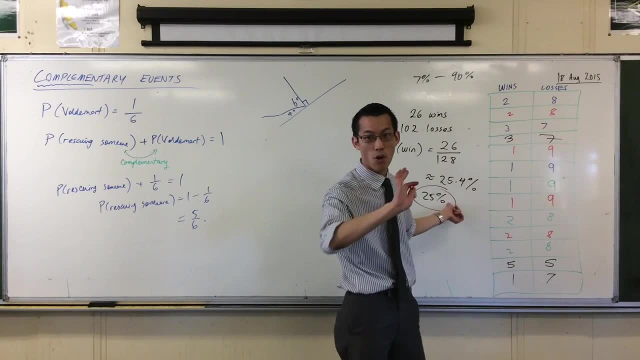 is it rounding up or down? I think it's rounding down 83,, 84,. okay, This is just to rescue one person, But this you've got to rescue all five, Right? So this is like. it's a bit like saying: 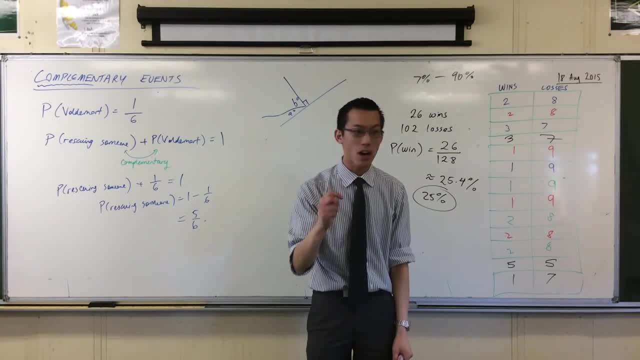 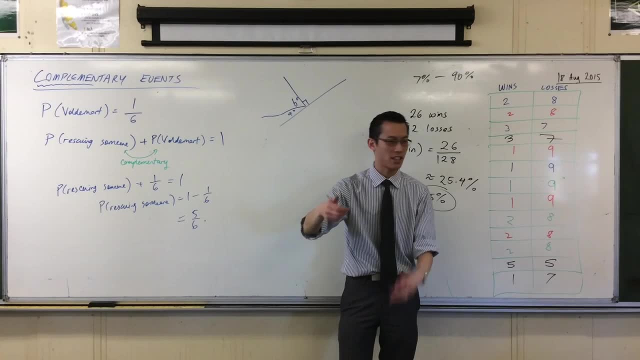 can you flip heads over and over and over again. It's not half, It's going to be a half, then it's going to be a quarter, then it's an eighth and then, however many heads you want to flip, then it's going to be less and less probable. okay, 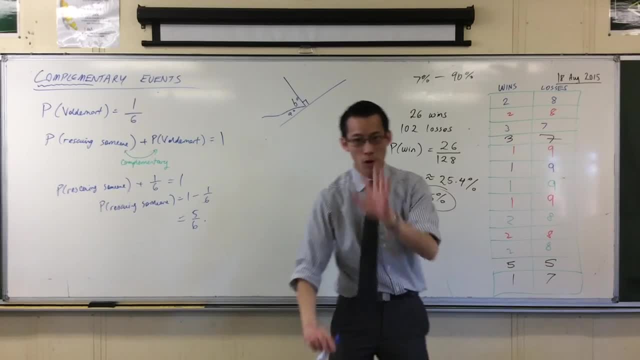 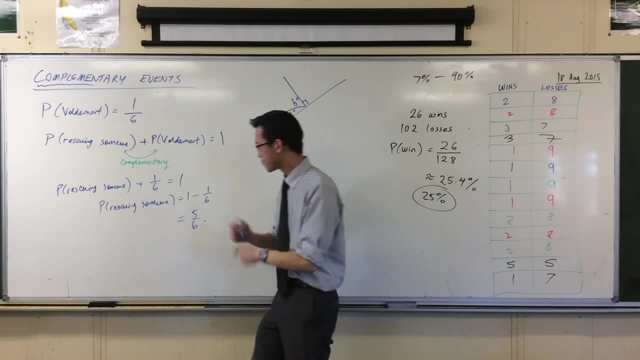 It comes down to a number like this: okay, So one more little bit of notation, Because this idea of complementary events, right, is very, very important. Let me abbreviate a little bit. Let's just call Voldemort V, okay. 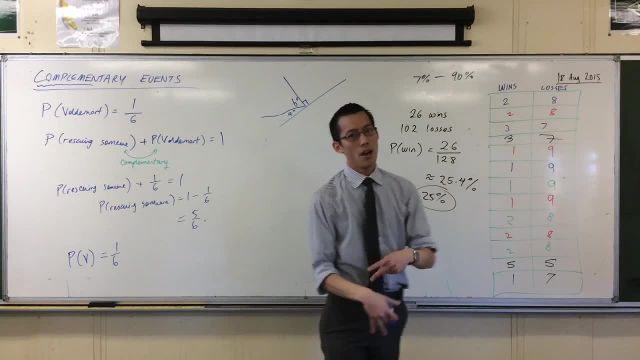 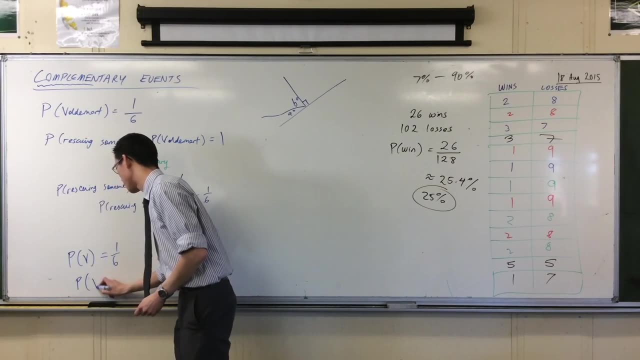 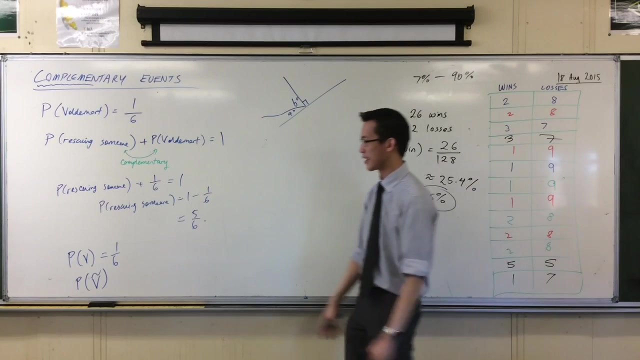 So the probability of V is one over six. okay, Because it becomes useful to talk about things happening or not happening, we introduce this little symbol here, which is a little squiggly line above whatever event you're describing. okay, It's like a tilt. 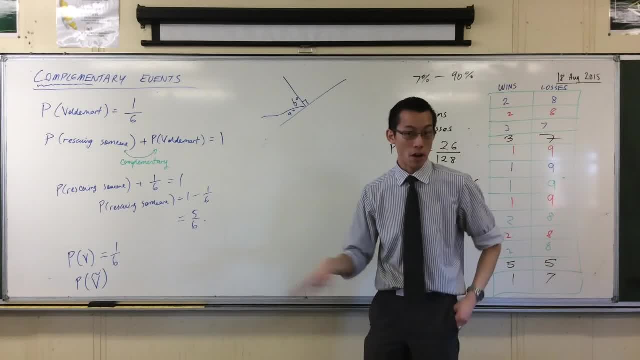 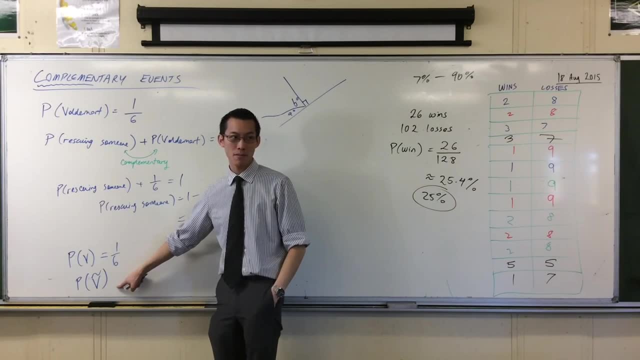 It is the same kind of symbol we use for estimate, but here what it means is complement, okay. So it's like: what's the probability of Voldemort killing you? What's the probability of him not killing you? okay. So this is like saying not, whatever that is. 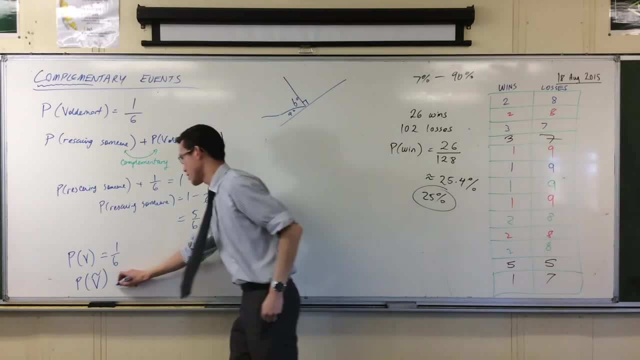 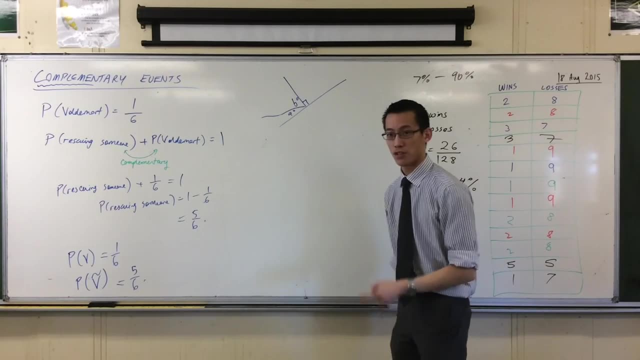 The opposite of whatever. that is The complement. So this is the same as this One. take away a six, It's five-six, okay. Now just be careful, Just before we set off on the exercise. we'll have about ten minutes, okay.